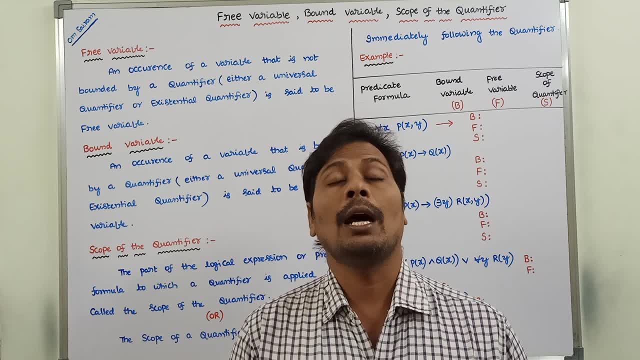 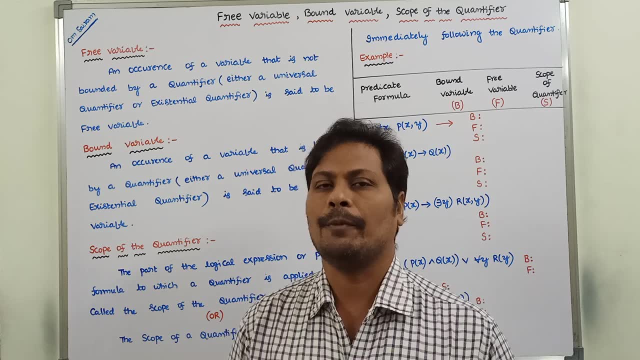 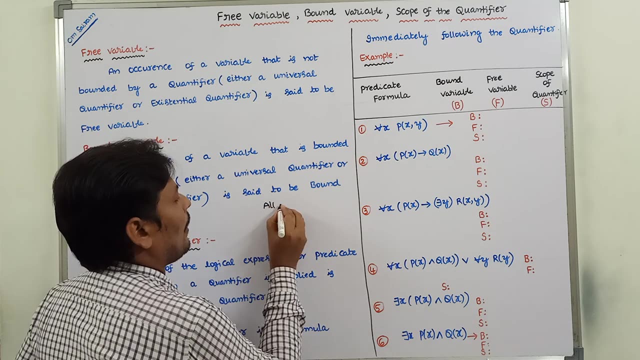 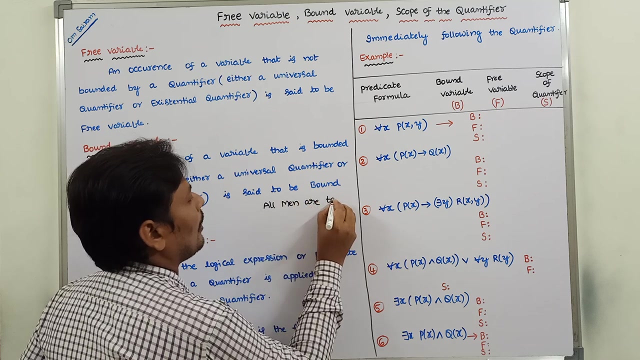 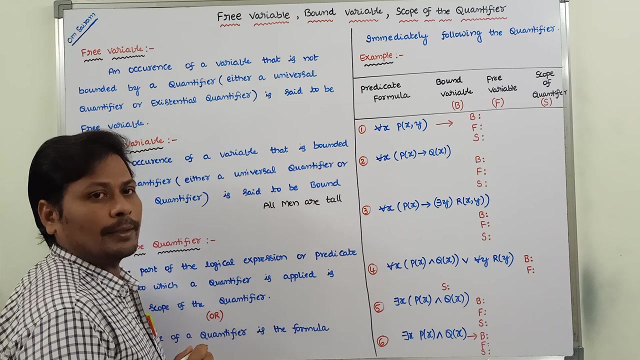 what is free variable, What is bound variable and what is the scope of a quantifier. So these are the points that we are discussed in this video. Okay, Suppose, for example, all men are tall. Okay, All men are tall, Okay. So this is the given statement. 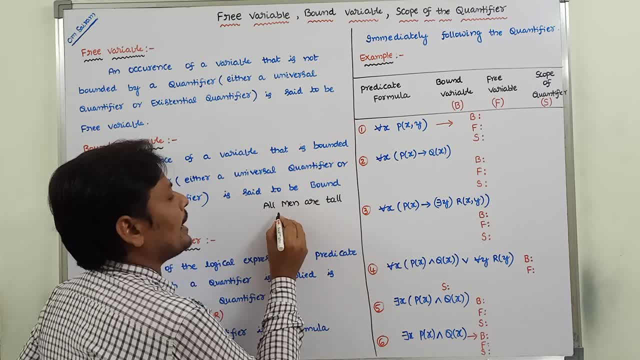 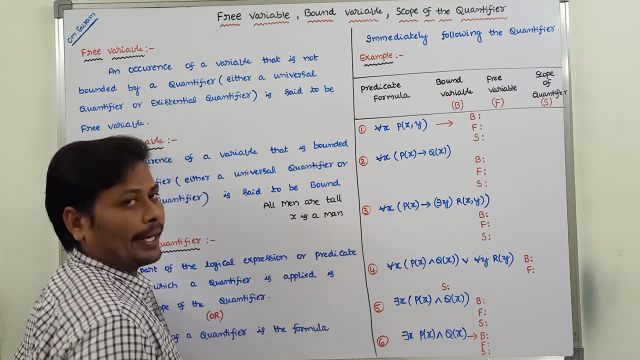 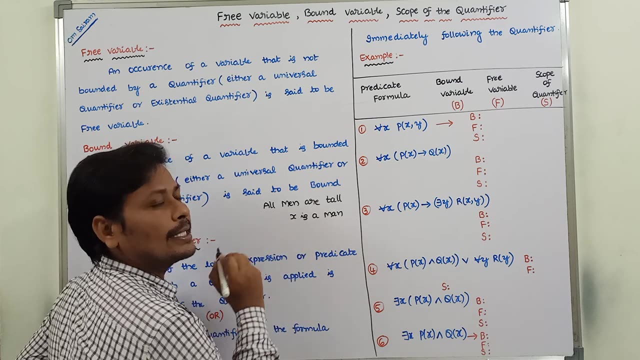 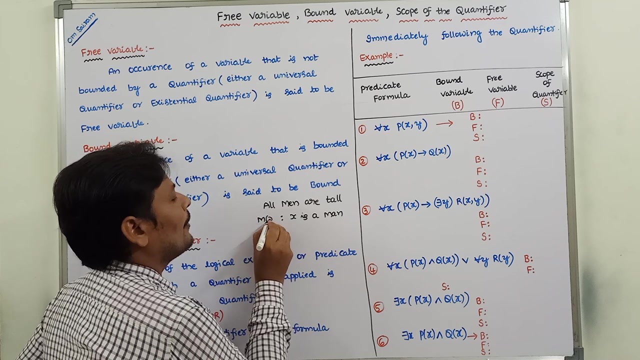 Okay, So this given statement can be written as: so: X is a man, X is a man. Okay, Here in this, one is a man, is a predicate and X is a subject over a variable, So it can be represented as M of X. 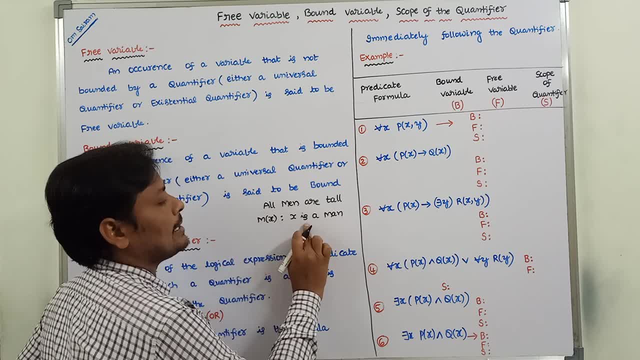 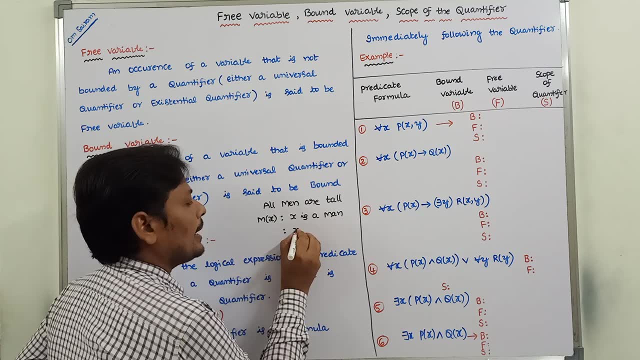 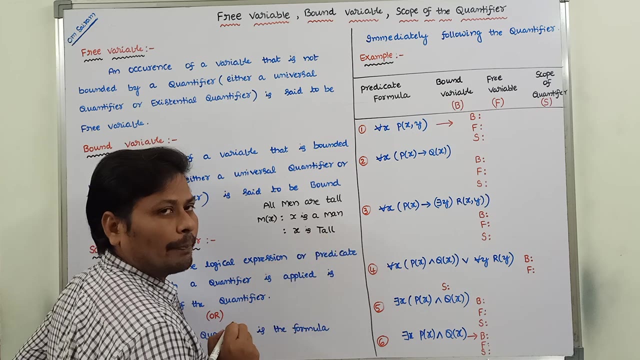 Here M is nothing but predicate, that is is a man, X is nothing but subject. Okay, In the same way. So x is tall, X is tall. So here is tall is the predicate, X is the subject. So is tall is the predicate. 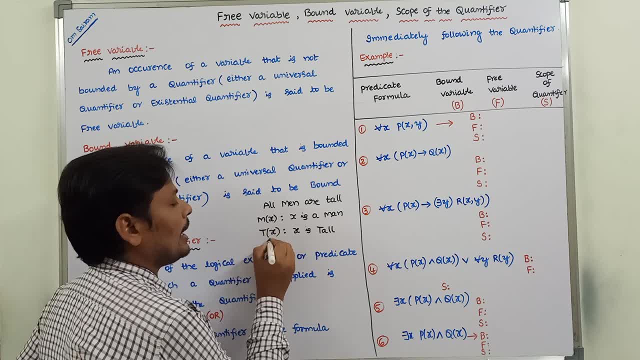 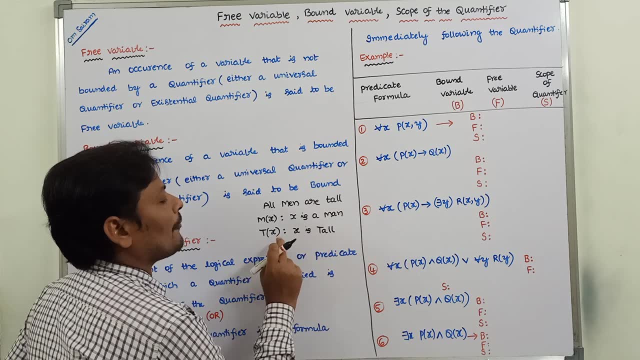 is denoted by capital T, So the subject is here X. okay, here M of X is nothing. but X is a man, T of X is the unaulos, So X is tall. So here as we go about this rest dream is: that is M of X is a man. Go back over and see. 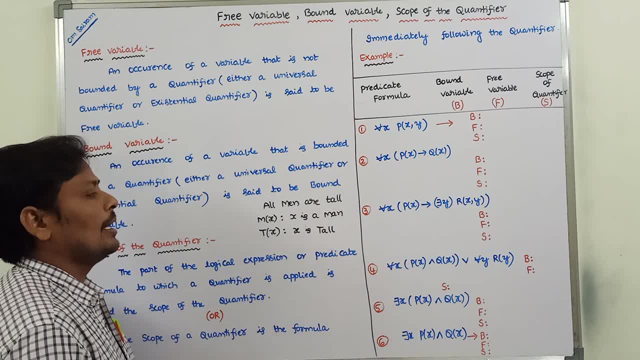 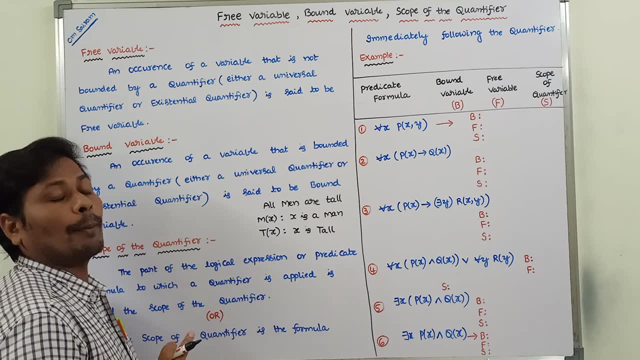 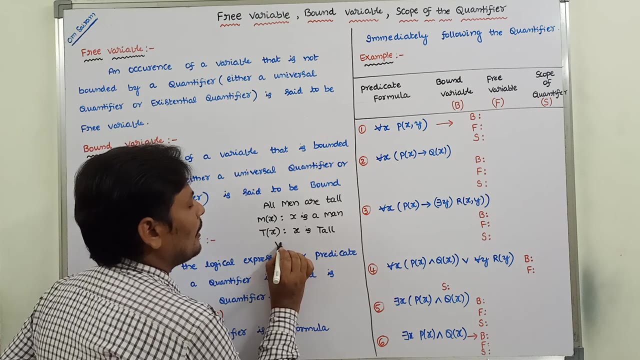 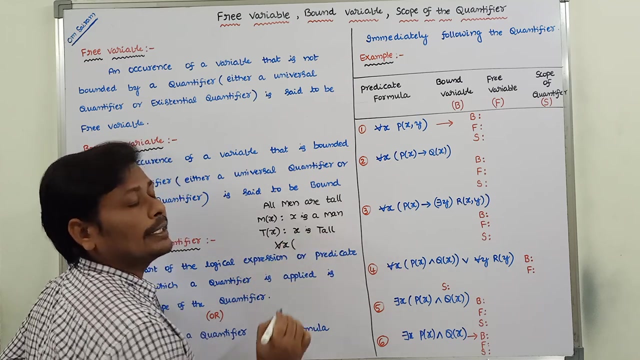 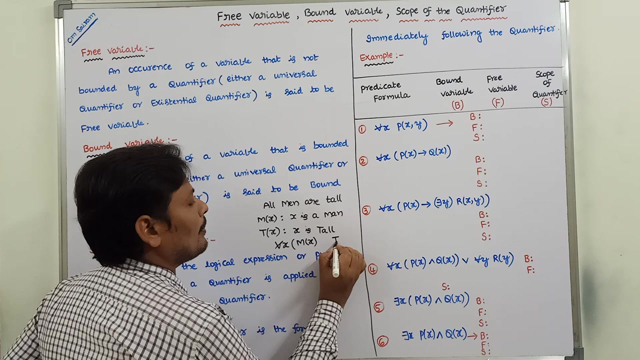 of x is x is tall. Okay, Here we now. we have to represent the above statement by using these two proposition functions or a predicate functions. Okay, So here it can be represented. as for all x, for all x, if x is a man, then x is tall. So x is a man means m of x. x is tall means p of x. 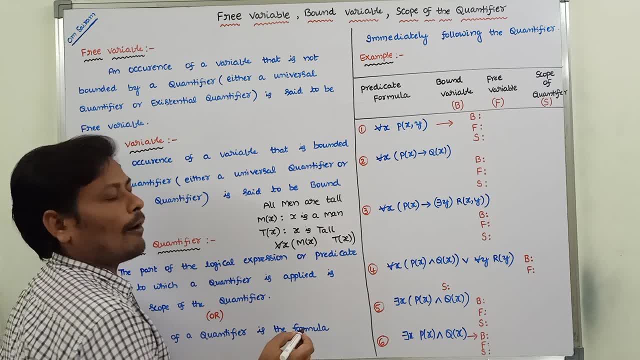 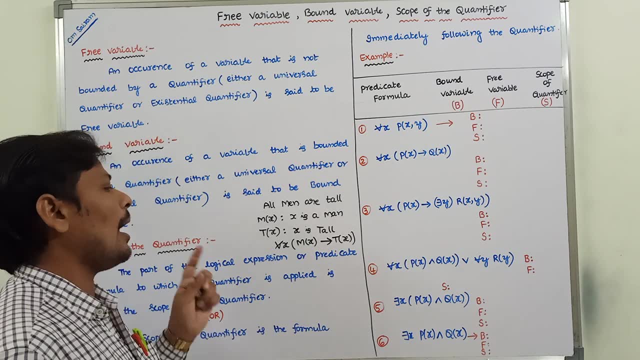 if x is a man, then x is tall. What is the connective in between them? That is conditional connective. Okay, So this is the. this is the statement that can be represented in a predicate function. Okay, So here we now. we have to represent the above statement by using: 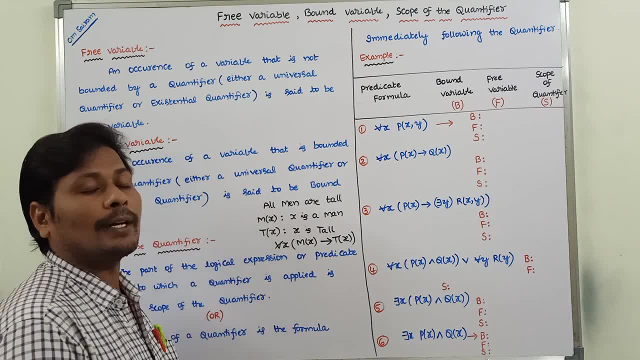 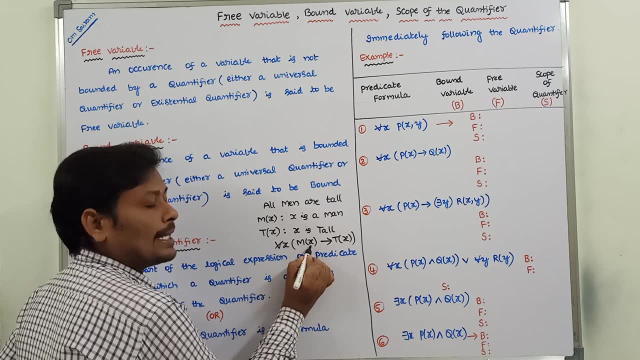 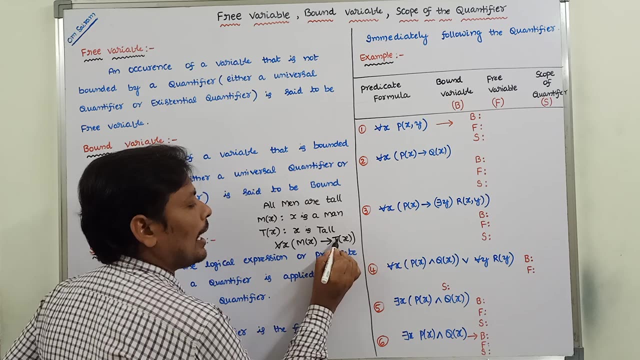 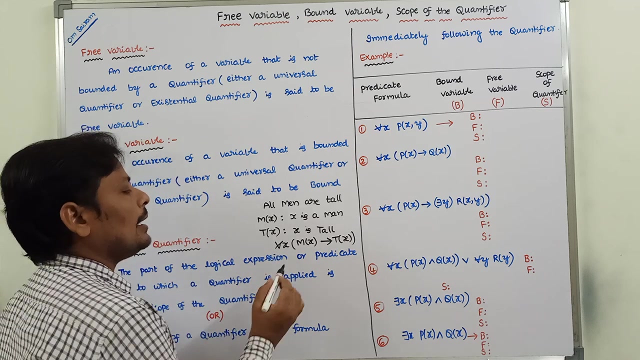 symbolic form by using universal quantifier. Okay, here, m of x is nothing, but x is the subject and m is the predicate. In the case of t of x, x is the subject and t is the predicate. Okay here. what is a bounded variable? Here the variable is x, An occurrence of a variable that is bounded. 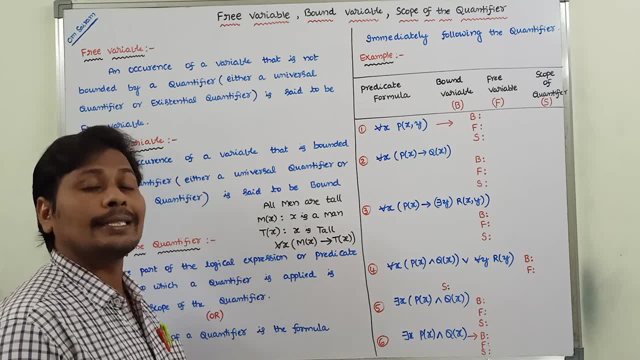 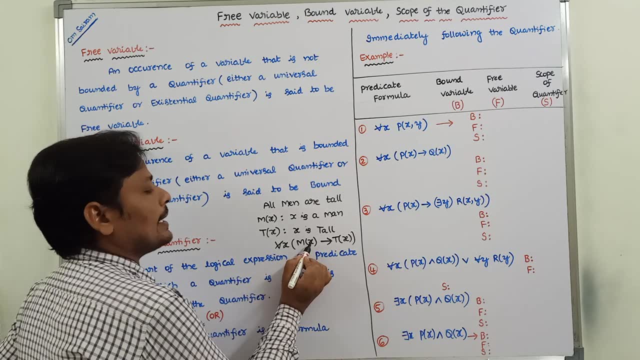 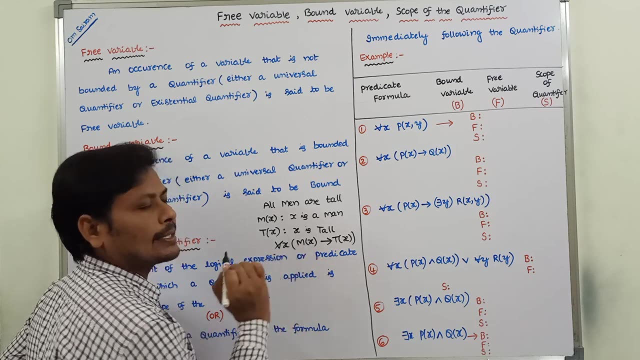 by either universal quantifier or existential quantifier, then x is called as bounded variable. Here x is the subject that can be also called as a variable. Okay, here, in this one x is the variable, x is the predicate. Okay, here, m of x is nothing. but x is the predicate. Okay, here, m of x is the. 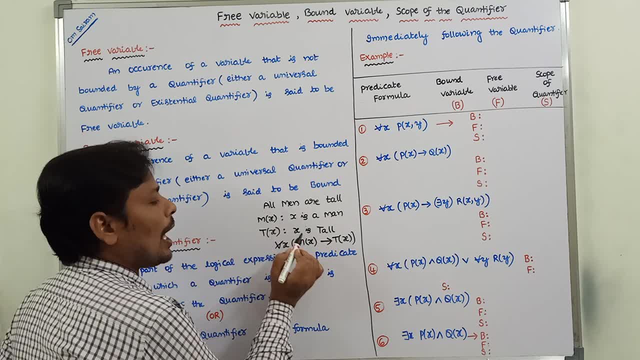 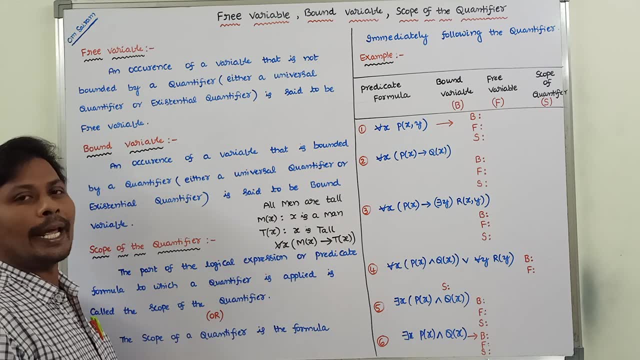 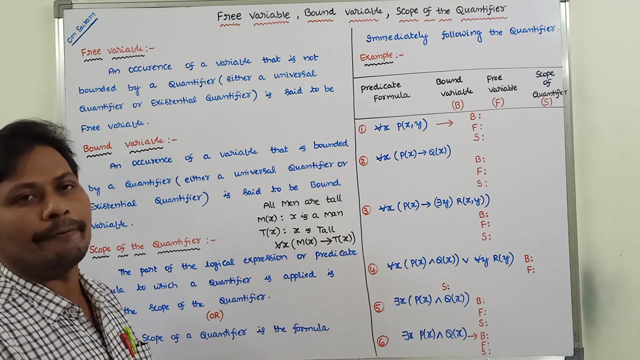 predicate. In this one, x is the variable. Okay, so now the variable x is bounded by either universal quantifier or existential quantifier. Here, in this case, the variable x is bounded by universal quantifier, then x is called as bounded variable. Okay, suppose for example: 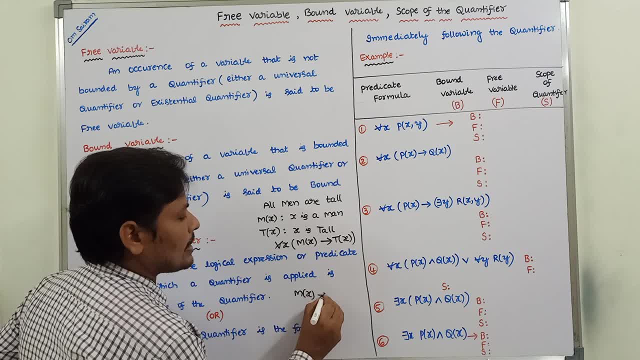 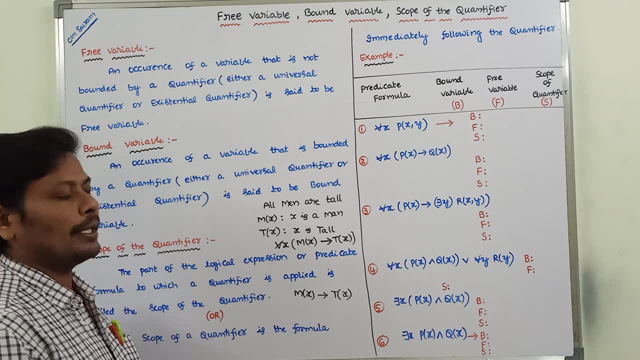 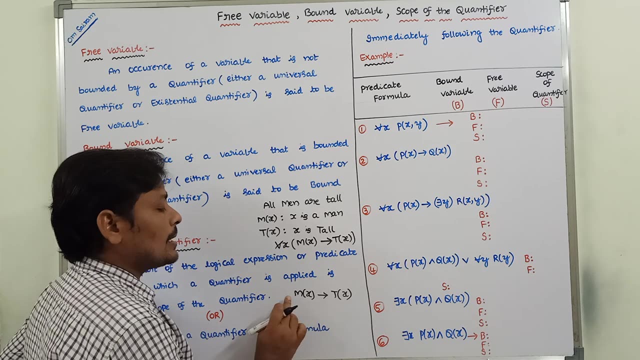 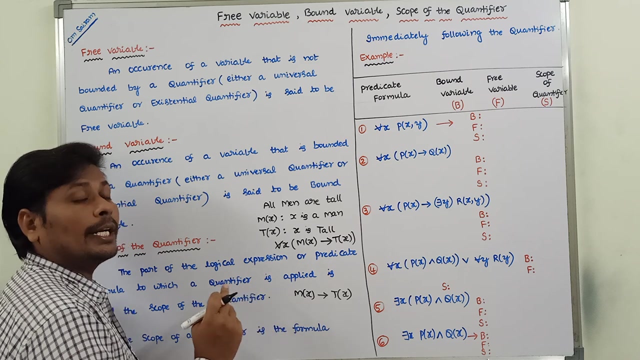 m of x. conditional t of x. Okay, so this is the symbolic representation of a particular statement Here: the variable x. okay, the variable x is not bounded by any universal quantifier. Okay, the variable x is not bounded by any universal quantifier or existential quantifier. 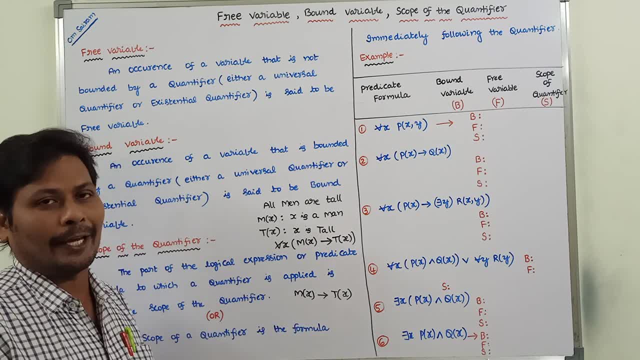 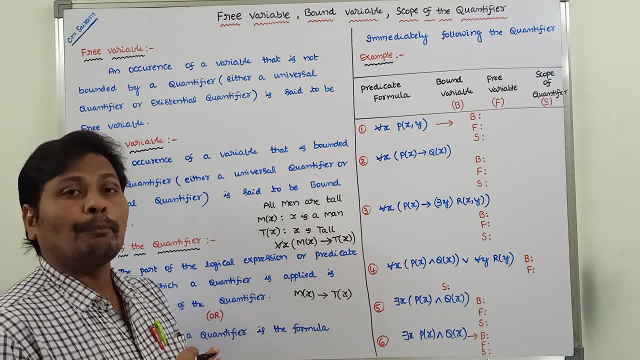 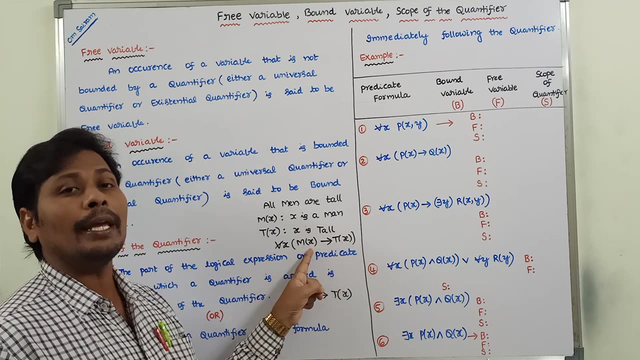 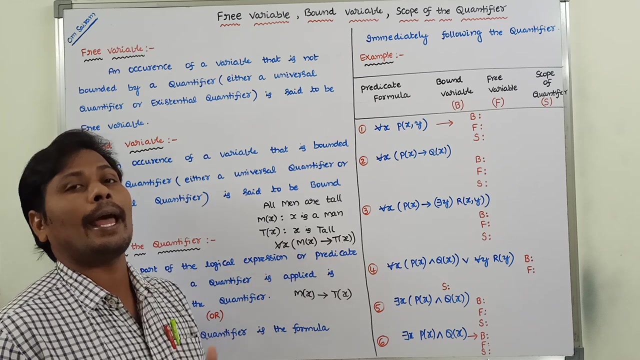 Then x is called as a free variable. Okay, so what is the difference between free variable and bound variable? An occurrence of a variable, an occurrence of a variable that is bounded by either universal quantifier or existential quantifier, then x is called as a bounded variable. 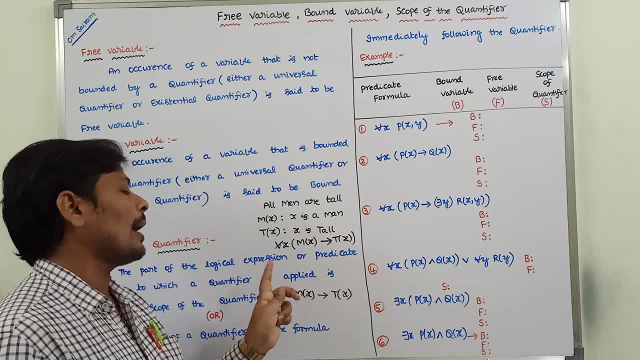 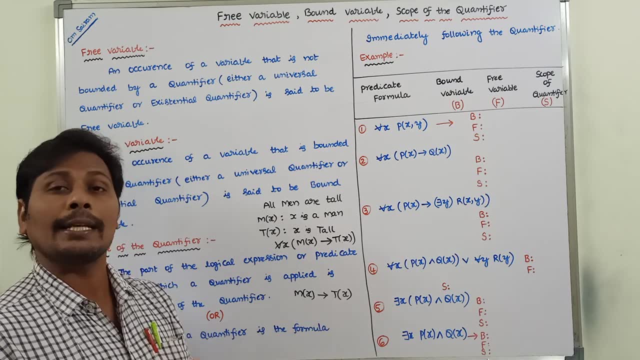 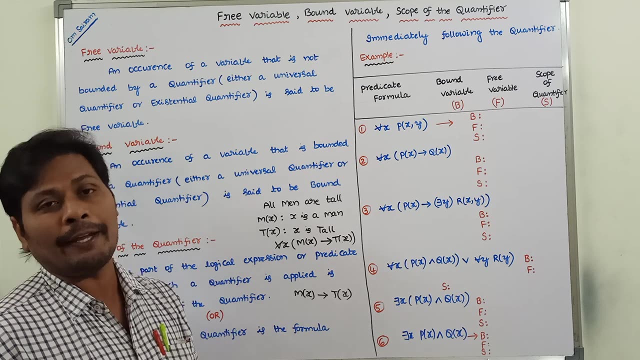 Okay, whereas in the case of free variable, an occurrence of a variable that is not bounded by any universal quantifier or existential quantifier, then the variable x or subject x is called as a free variable. Okay, so next one, what is the scope? 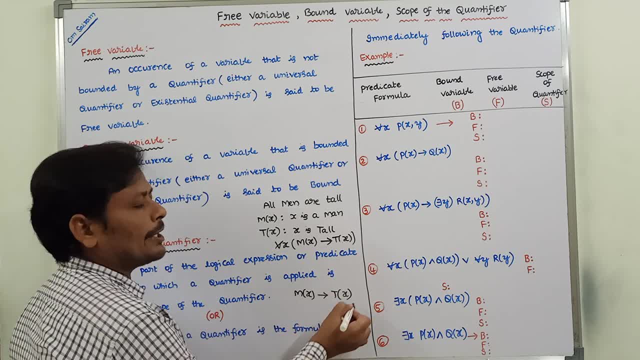 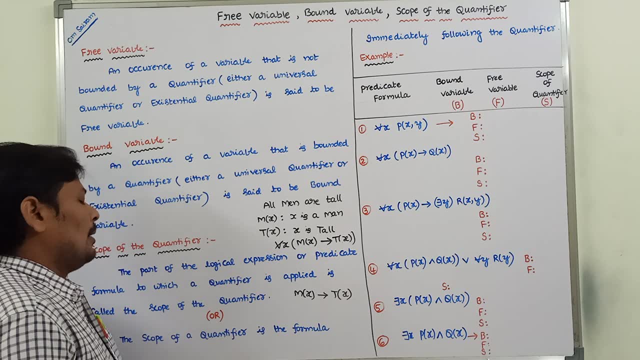 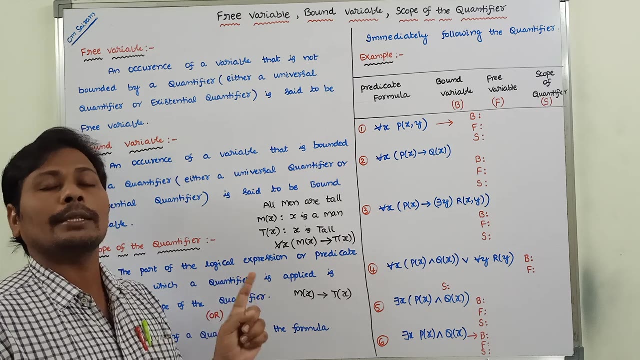 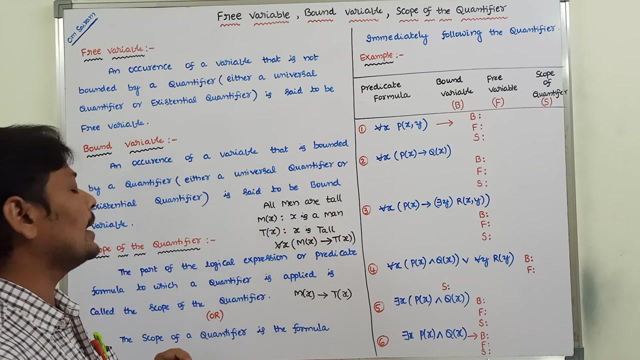 of a quantifier. Okay, so this is one predicate formula. This is one predicate formula and this is also a predicate formula To which a quantifier is applied. Okay, a predicate formula, or the part of the expression to which a quantifier is applied. so then it is called as a scope of the quantifier. Okay, so simply we can. 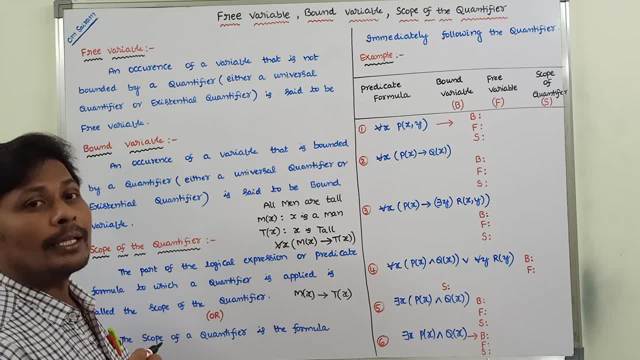 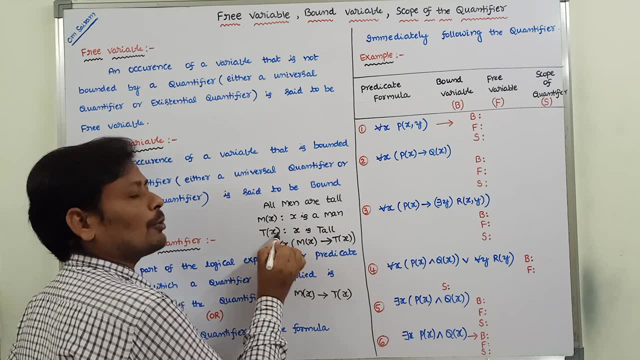 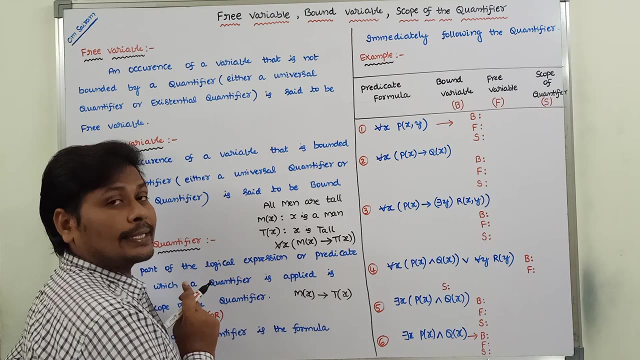 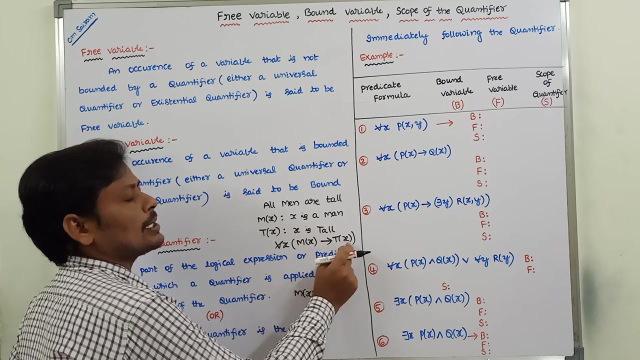 say that the scope of a quantifier is the expression that immediately follows the quantifier. Okay, what is the expression immediately followed by the quantifier? So here for all, x is the universal quantifier. This is the expression or predicate formula m of x. conditional t of x. Okay, so the 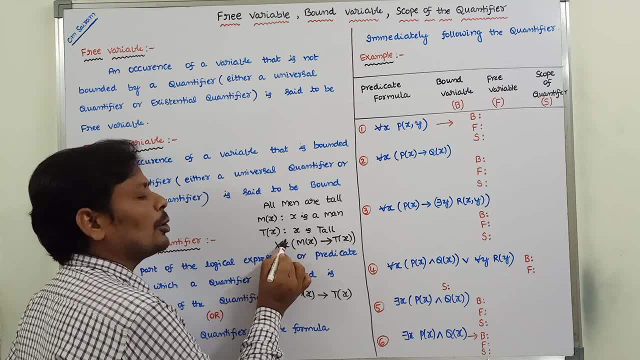 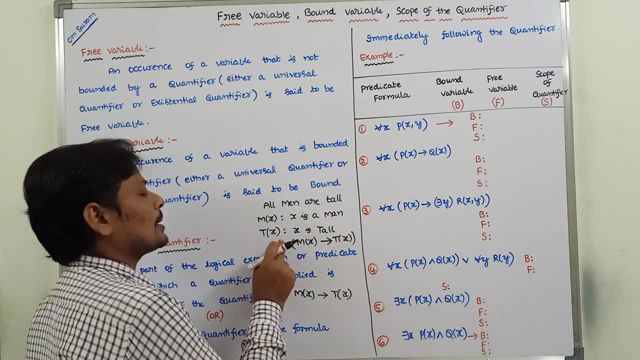 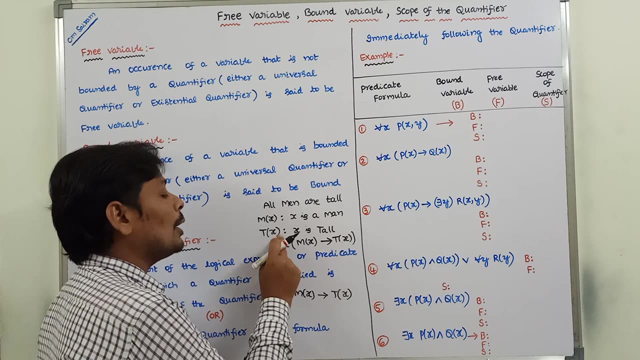 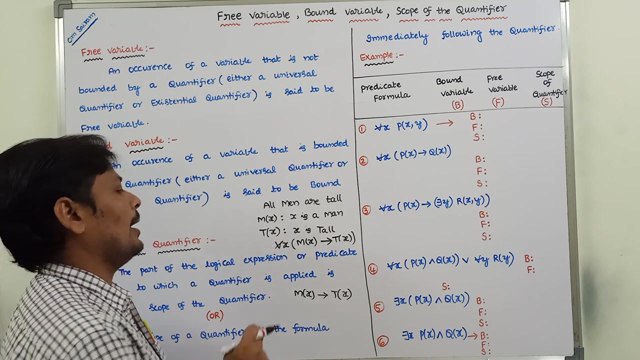 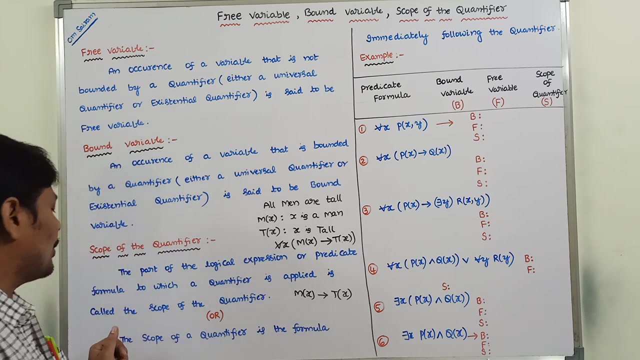 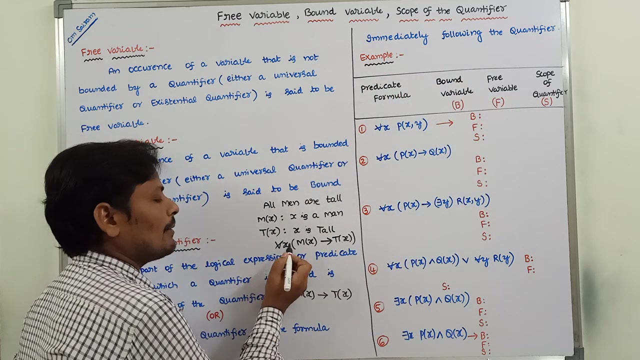 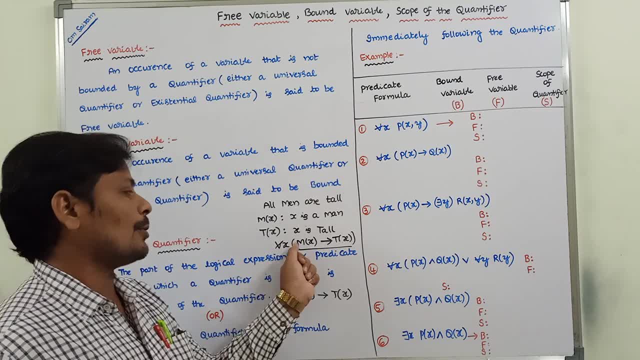 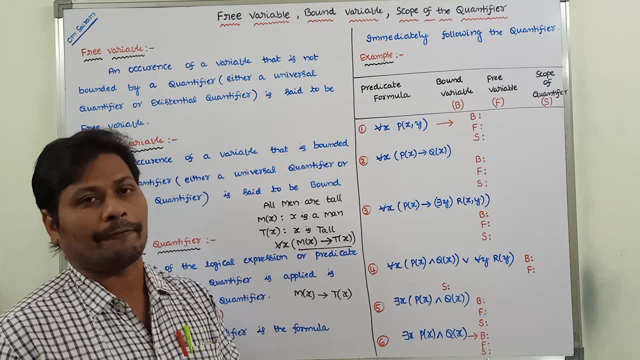 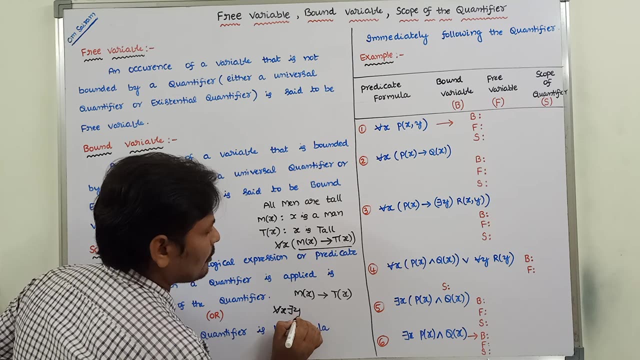 m of x conditional t of x. So now m of x. conditional t of x is the scope of the quantifier, that is universal quantifier. Okay, for example, for all x there exists y. So M of X conditional T of Y. 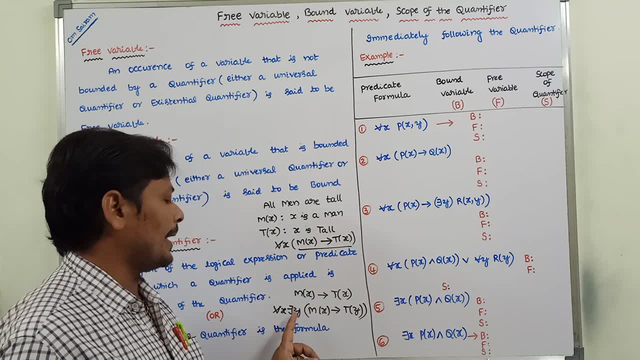 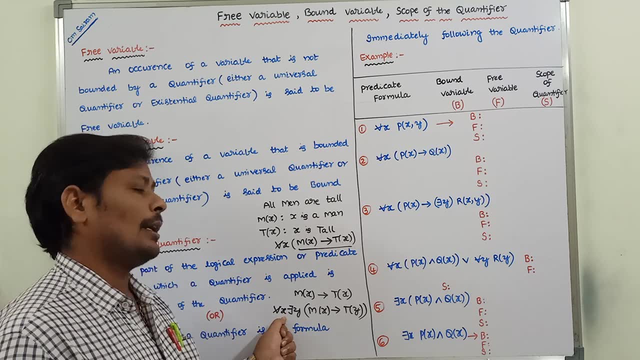 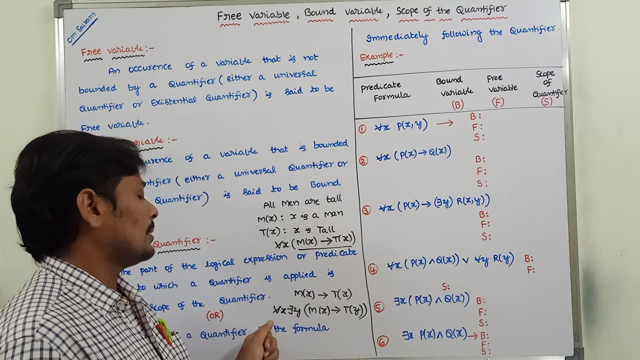 Suppose this is there For all X. there exists Y, M of X, conditional T of Y. So what is the scope of the universal quantifier? The scope of the universal quantifier is M of X conditional T of Y. There exists Y, M of X, conditional T of Y. 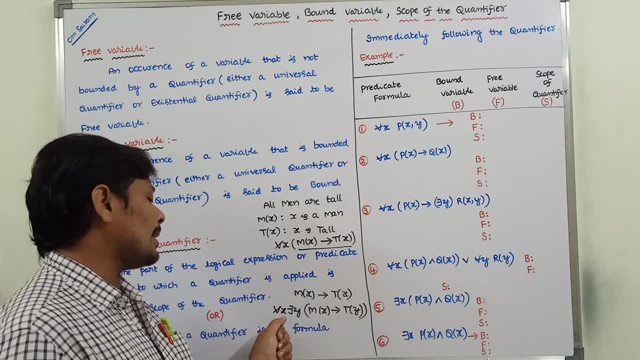 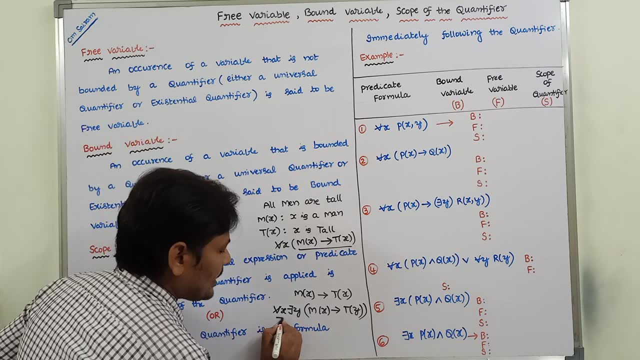 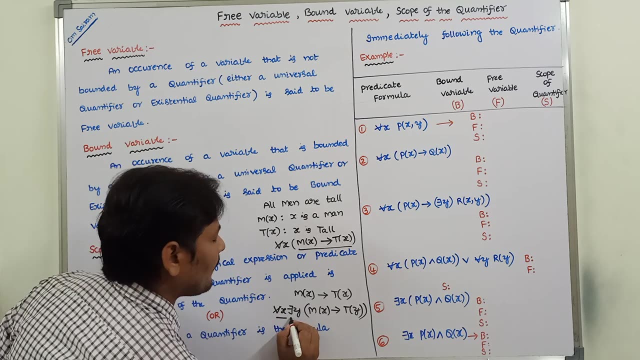 This is the scope of the universal quantifier. What is the scope of the existential quantifier? M of X? conditional T of Y? Okay, here, this is the universal quantifier. The expression that immediately followed by the universal quantifier is called as scope of the quantifier. 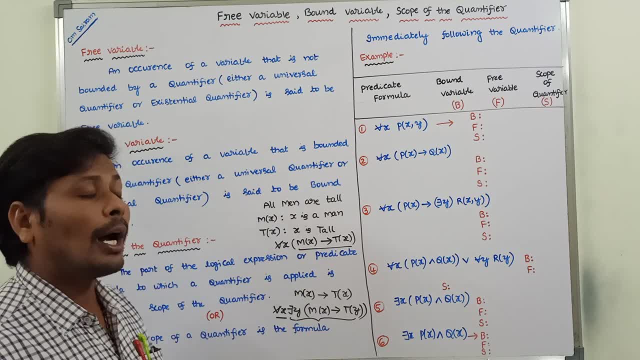 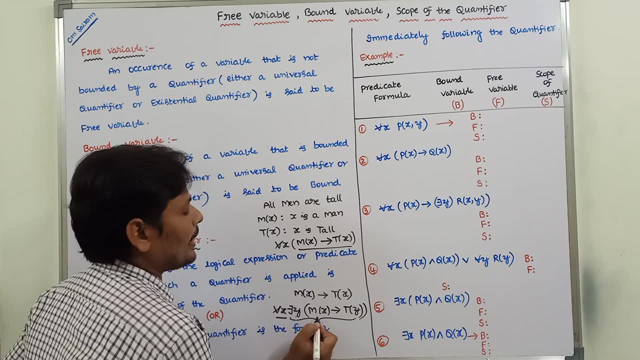 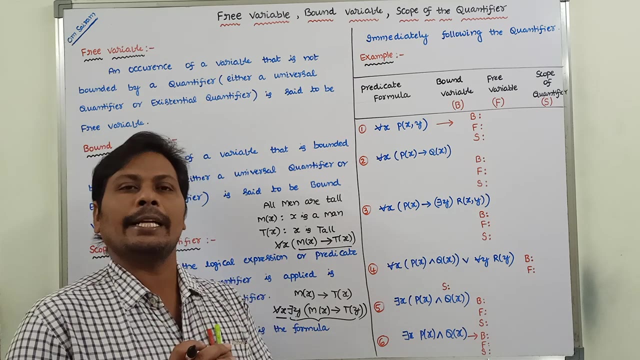 There exists Y, M of X, conditional T of Y. What is the scope of the existential quantifier? is So the expression? The expression immediately follows the quantifier is M of X, conditional T of Y. Okay, So the simply we can say that what is free variable? 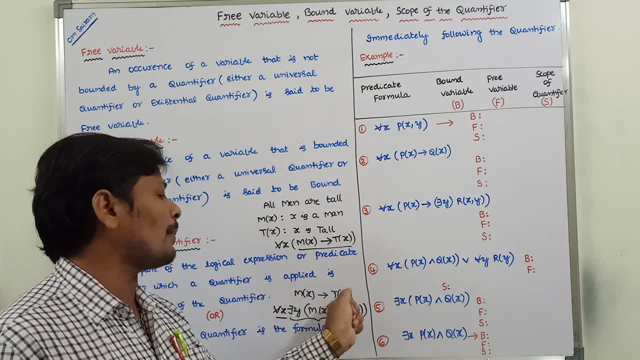 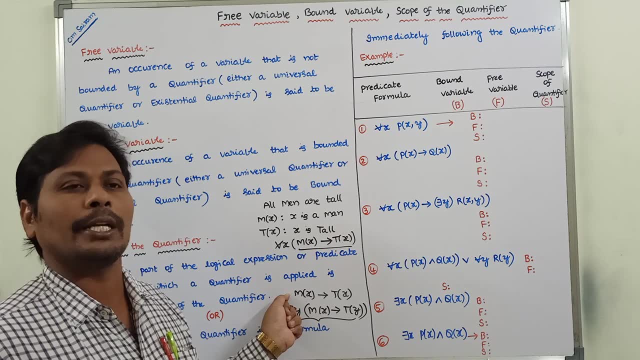 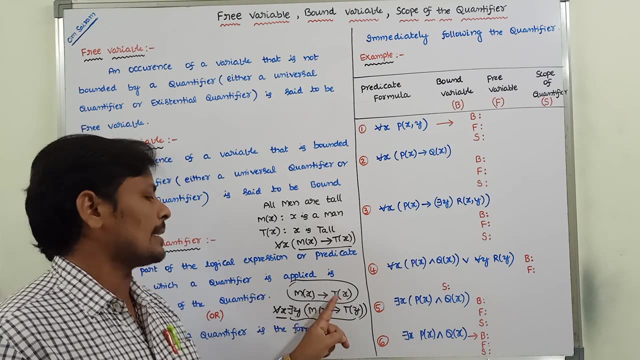 An occurrence of a variable that is not bounded by any quantifier, either a universal quantifier or an existential quantifier, Then it is called as a free variable Here. in this case, the variable X is Not bounded with any quantifier. 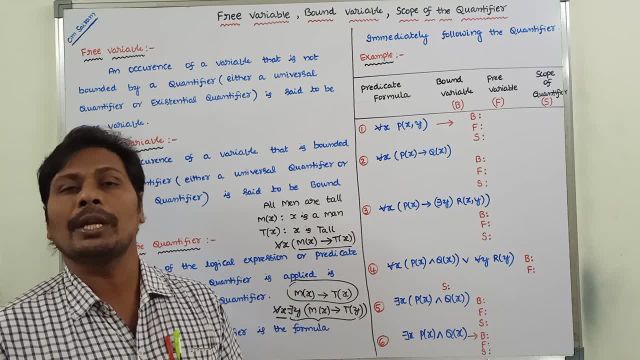 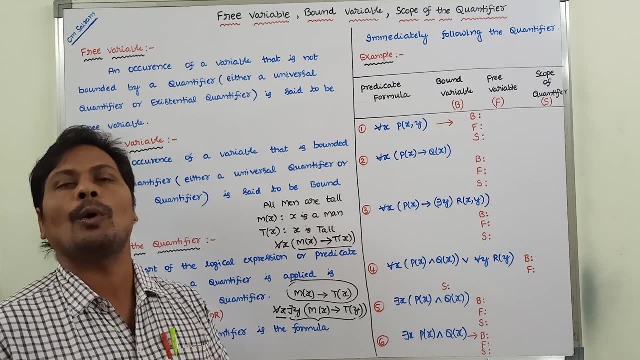 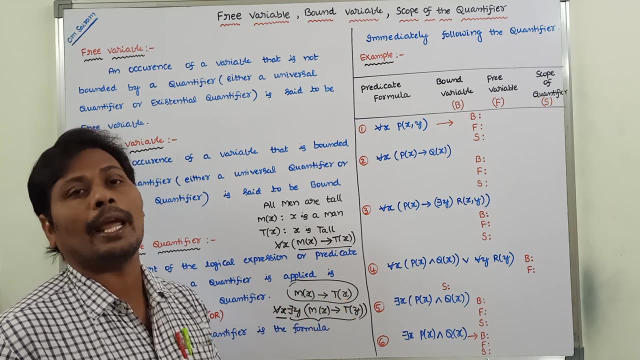 So hence the variable X is called as a universal quantifier. Okay, Variable X is also called: here is subject: Okay, Subject over our object over our variable. Okay, So the variable X is not bounded with any quantifier, either a universal quantifier or a existential quantifier. 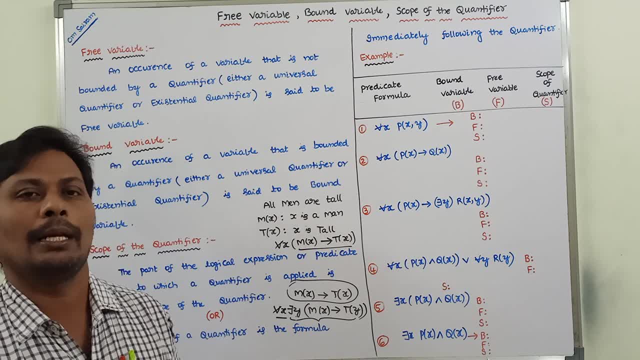 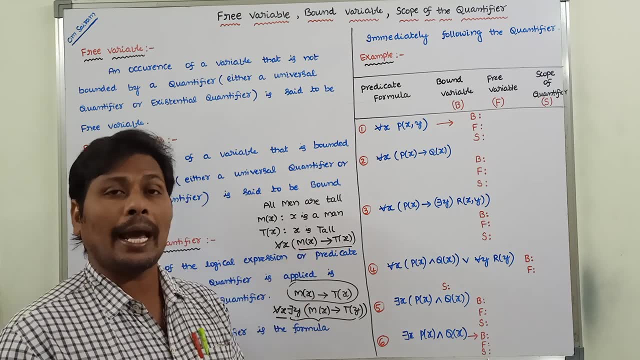 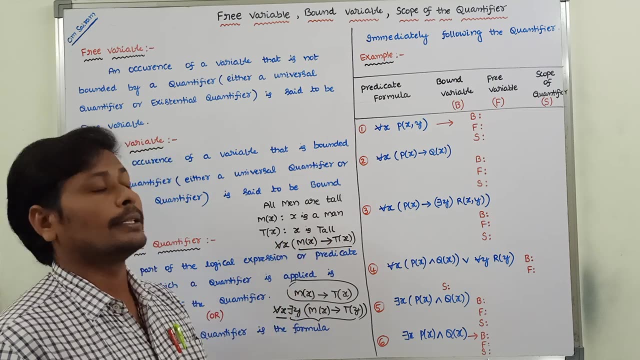 Then X is called as a bounded variable. Okay, X is called as a free variable. Okay, Here, in this case, the variable, the occurrence of a variable, is bounded with a universal quantifier. Then the variable X is called as a bounded variable. 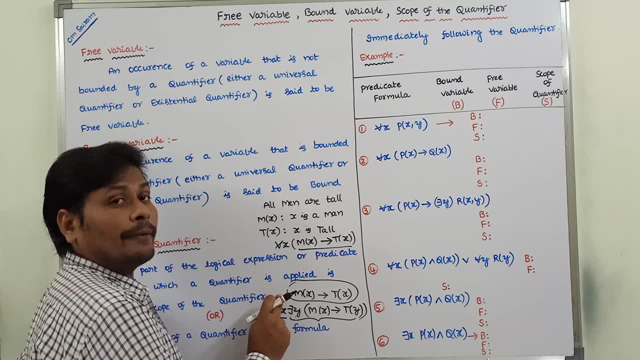 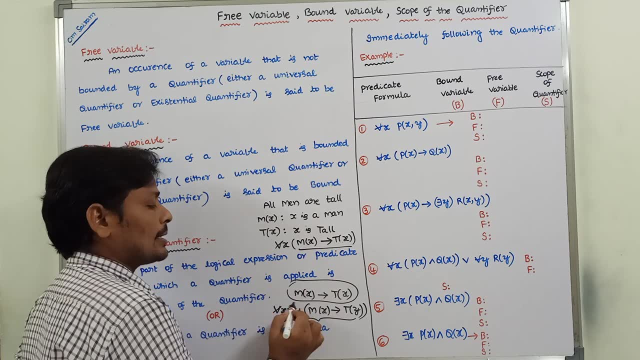 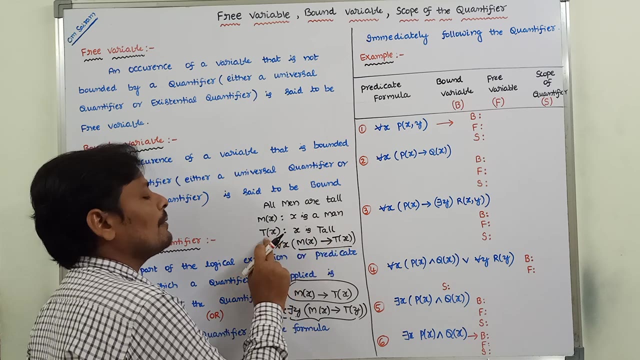 Here the variable X is not bounded with any quantifier, either a universal quantifier or a existential quantifier, Then X is called as a free variable. Here, in this case, the variable X is a bounded with a universal quantifier, Then X is called as a bounded variable.